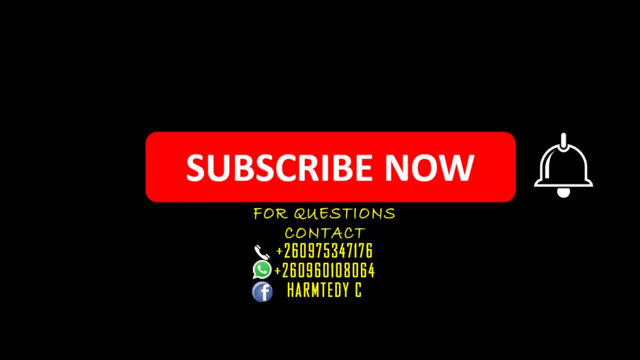 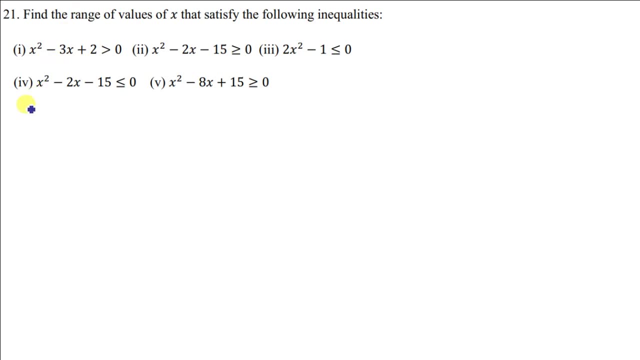 and the notification button and if you have any questions, feel free to contact me on any of the lines on the screen. So let's see how we can solve these questions. So the first thing that we need to find, when you've been given such a question, you need to 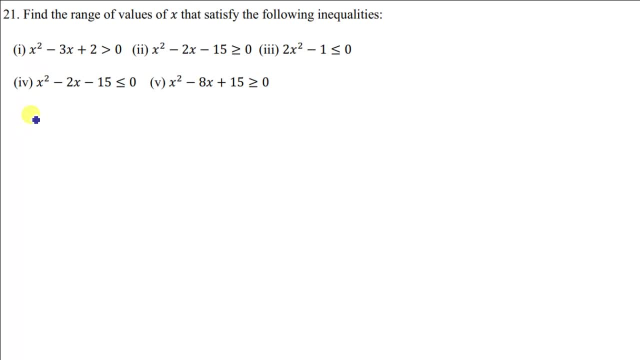 find what are known as critical points. So we have the question: is x squared minus 3x plus 2.. So to find critical points, we equate these to zero. I mean, we equate the equation to zero. So I'm going to factorize this equation. So the product for this equation 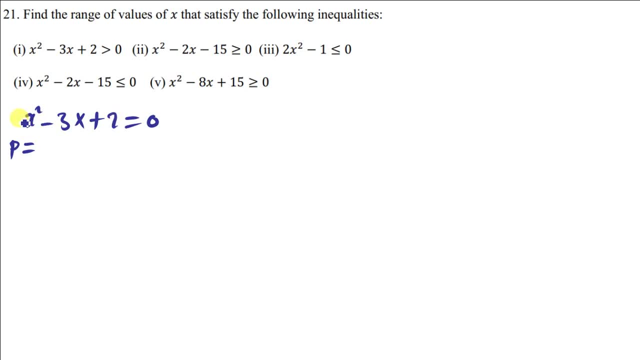 is simply just going to be found by multiplying the coefficient of x squared and the constant 2 times 1. we'll get 2.. Then the sum is going to be found by just getting the coefficient of x, which is negative 3.. Okay so, the factors of the product, that if we multiply them we'll get 2, and if we 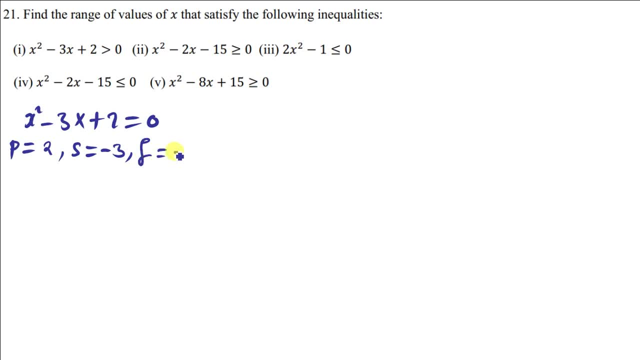 add them, we'll get negative 3.. We are simply just going to get negative 1 and negative 2.. So when you multiply the 2, you get positive 2.. When you add them, you get negative 3.. Okay, so let us now replace the factors while there's negative. 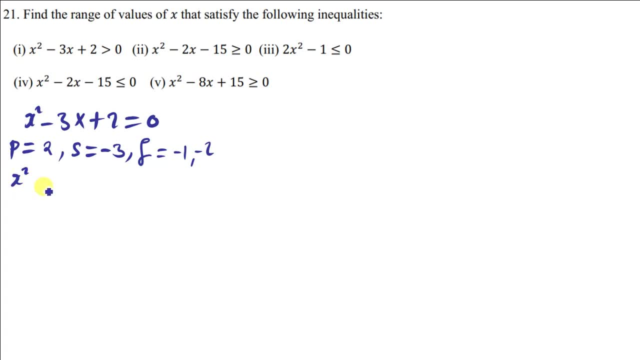 3 there. So we have x squared. then we have negative x and then negative 2x. Then we have positive 2 there. So this is equal to zero. So we open the brackets. there we have x minus 1. then we factorize there also have x minus 1.. 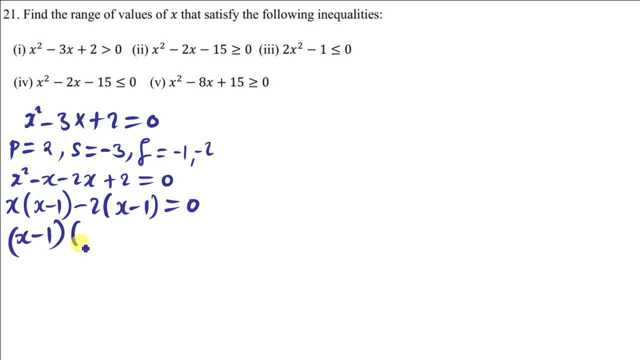 Then we're going to have x minus 1 there and x minus 2 there, So this is equal to zero. So when you equate both the factors to zero, we're going to get x minus 1 is equal to zero and x minus 2. 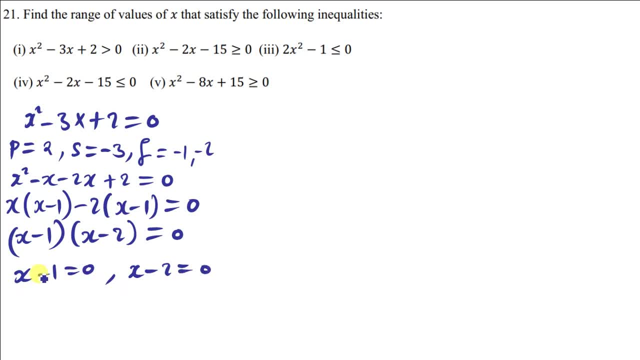 is equal to zero. take this negative one to the other side of the equal sign: you get x is equal to positive one. then you take this negative one to the negative two to the other side, you get x is equal to two. so these are known as- uh, the critical points. so these are not the final solutions, but these are. 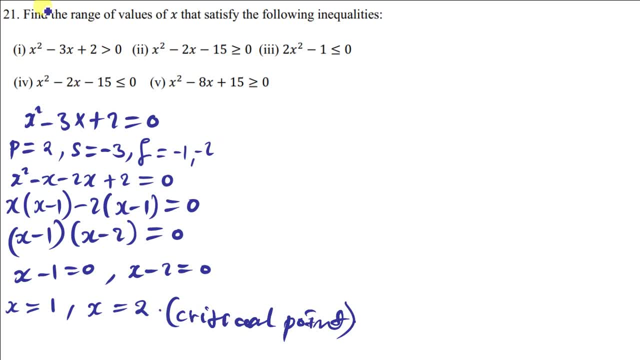 just points that we're going to use to test to find the range of values of x. so i'm going to draw a simple number line here where i'm going to put my critical points. so the two critical points i have are one and two. so these numbers that are this side are going to 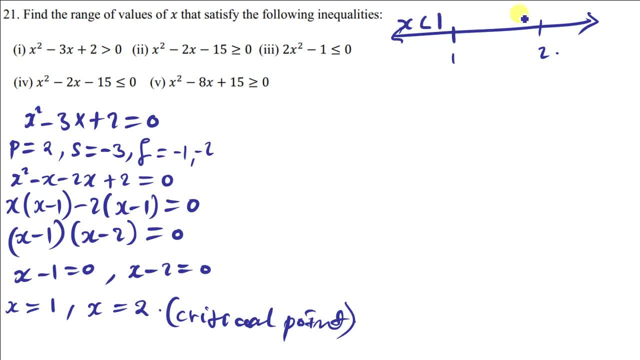 say: these are values of x that are less than one. the numbers in between are values of x between one and two. then numbers this side are values of x that are greater than two. so i'm going to write the same equation and put back the symbol there. 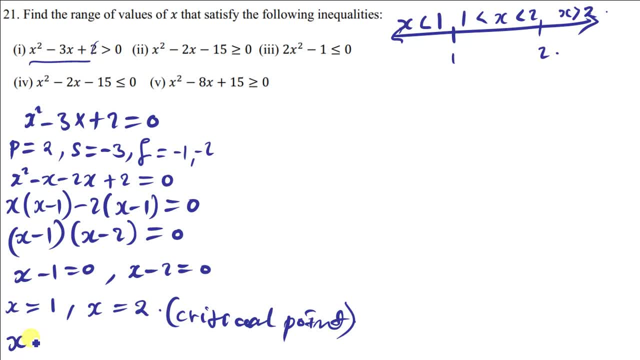 which is the greater than symbol. so, oh sorry, i'm instead. i'm supposed to write this, so i'm not supposed to write this. i'm supposed to write this expression, so let me just write it here, so i'm having x minus. you can even use this same one, there's no problem, but i prefer using this one. 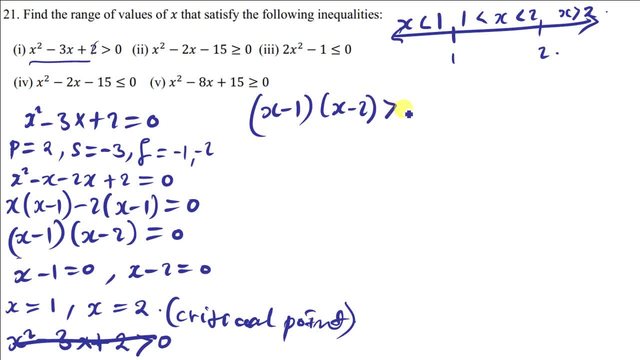 then i'll put this symbol, which is a greater than symbol, so i'm going to get any number that is less than one, uh, so in this case i can even get zero, so you know. so when i get that zero, i'll replace it. black is x to test to find if this region will be. 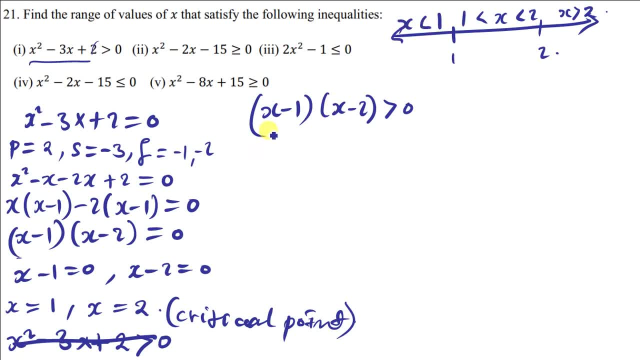 accepted. if it's part of the range of values of x, is x equal to 0.. so again, so i get the zab forum x, so we can put a 0 there. 0 minus 1, we're getting negative 1. so negative 1 is a negative number. i'll. 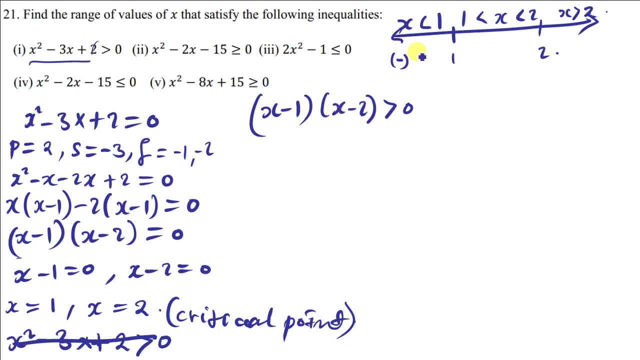 just write a negative there and then 0 minus 2 also give us negative 2. it's also a negative number. i'll just write a negative. negative times negative gave us a positive. so is a positive number greater than 0 following this symbol here? is it greater than 0? the answer is yes meaning. 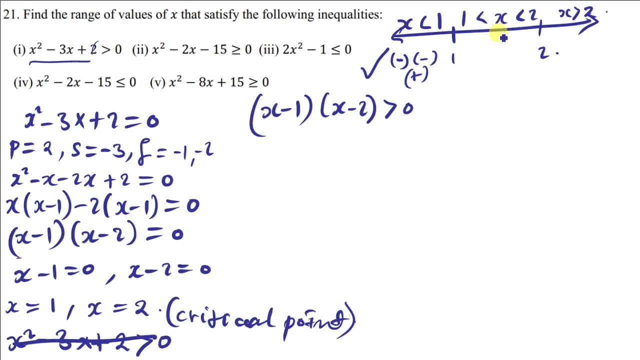 this is one of the ranges of values of x that we're looking for. okay, so we also get any number between 1 and 2, so we can get 1.5 when you put 1.5 here, where this x have 1.5 minus 1, the answer. 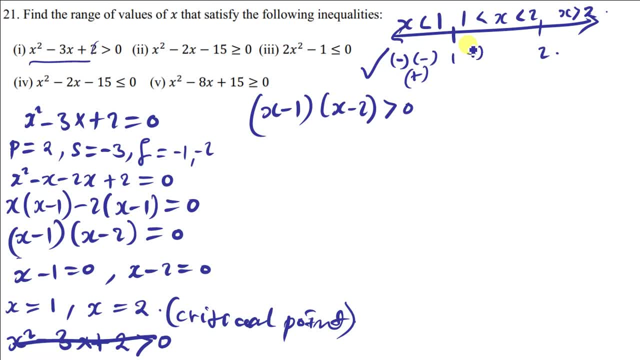 is 0.5, which is a positive number. so i'm going to put a positive number there, i mean a positive symbol. then 1.5 minus 2 give us a negative answer. so we put a negative there. so negative times positive. the answer is 0.5. so we're going to put a positive number there and then 1.5 minus 2. 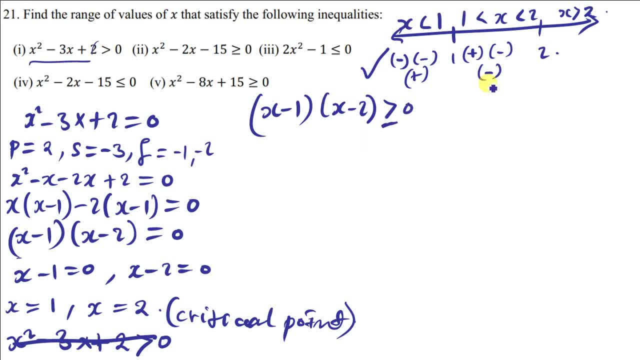 the answer will be negative. is a negative number greater than 0? the answer is no, and if the answer is no, meaning this region is not part of our solutions. so we get any number that is greater than 2. so any number that is greater than 2, we can even get 3. so when you put 3 where there's x, 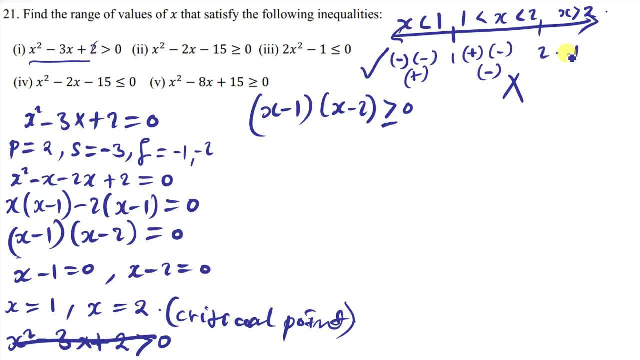 there. i'm going to have 3 minus 1. the answer is positive 2. so i'm going to put positive 2 there and then 3 minus 2, the answer is positive as well. so you put a positive symbol there. positive times, positive, the answer is positive. 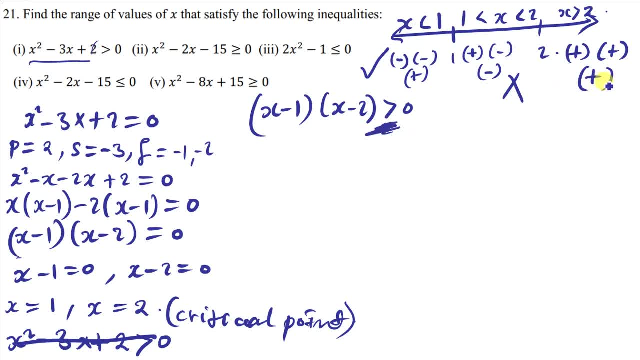 so it's a positive number greater than 0? the answer is yes, so the two regions that we're looking for, which will satisfy this inequality, are simply just x less than 1 and x greater than 2. these are the two regions that we are looking for. okay, so i'll also pick another question. 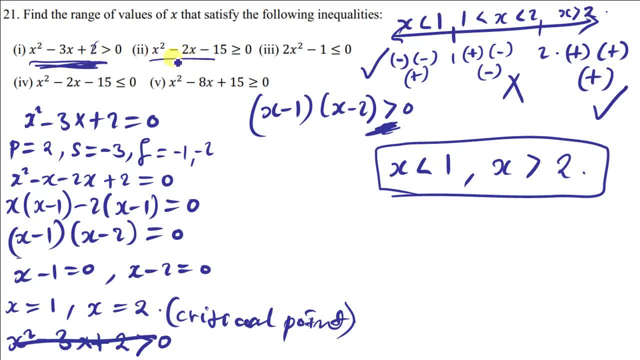 so, the same way i've solved this one, it's the same way you solve this one. the first thing you find the critical points. then, after finding the critical points, you test them in the region. so make sure that if there is a greater or equal to symbol, or less or equal to symbol, even these you just 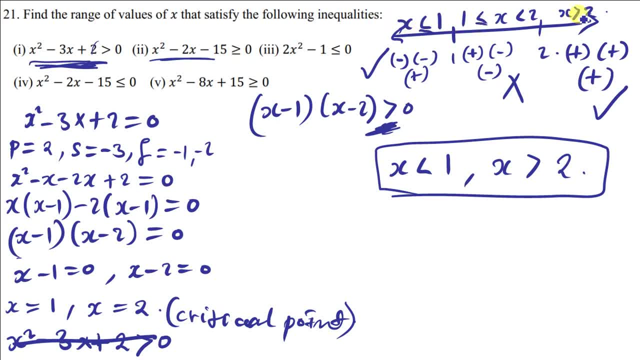 you put equal symbols like that, so meaning the solutions should also have the less or equal to, or greater or equal to symbols. yeah, so that's the only difference between this one and this one. yeah, otherwise you find the critical points and also put them on the number line, like that. so let's. 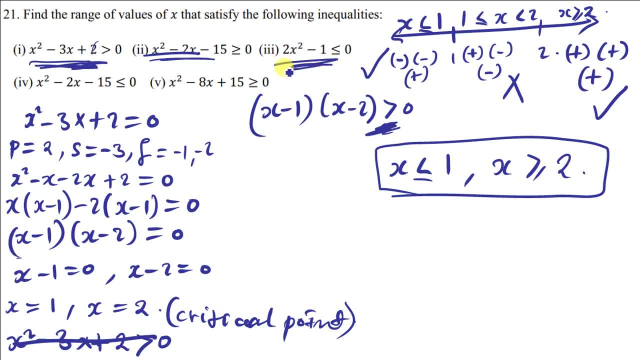 take a look at how we can find this one. so the same: I've found this one. it's the same way you find this and also this one. let me just solve this one. so if, if you want, you can solve the questions which I've left- this one, this one and that one- then submit the. 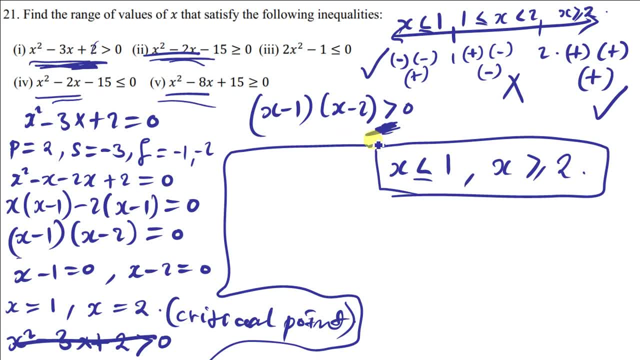 solutions using my WhatsApp line, then i'll help you. I'll tell you whether your solution is correct or wrong. so this is what we have. so take this before we take it. we take negative 1 to the other side of the equal sign. the first thing that we need to do is to equate this to 0, so we're. 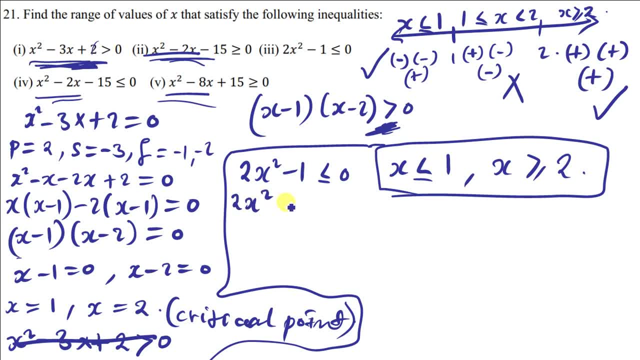 going to say: 2x squared minus 1 is equal to 0. so we have done this so that we can find the critical points. so you take this negative 1 to the other side of the equal sign and then let her divide by 2, so you're going to get x squared is: 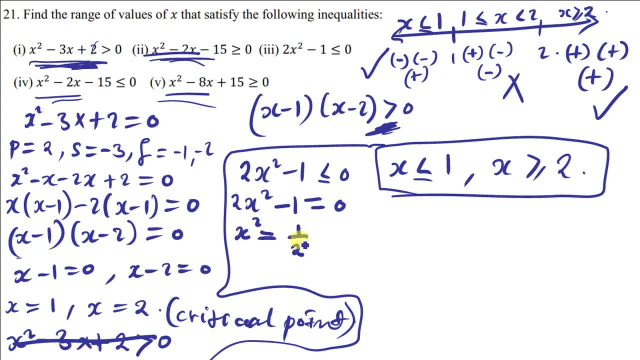 equal to 1 over 2. then to find the critical points, you say X. you find the square root of both sides, this side and this side. of course this should be plus or minus. so the value of X will be plus or minus the square root of 1 over 2. so 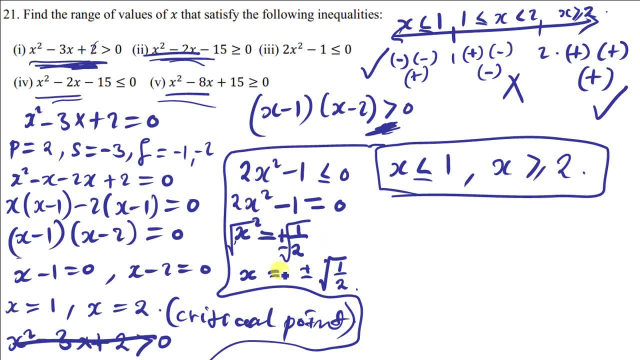 I'll take this negative, so we have taken the negative 1 to the other side of the. So these are some of. I mean these are the two critical points that we have, So we take them on the number line So you can also write them as plus or minus 1 over the root of 2.. 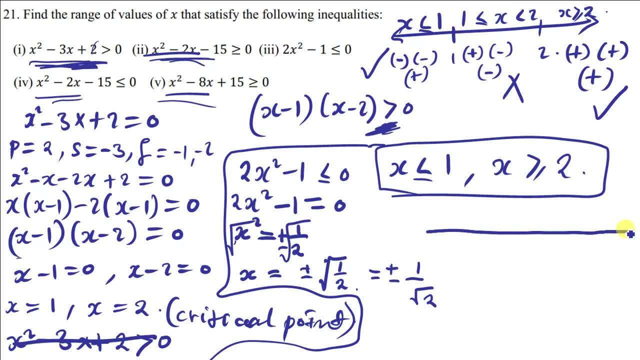 So what you just do is you just put them on the number line, So you have negative root 1 over 2 and also positive 1 over root 2.. So this side you have x less than negative 1 over root 2.. 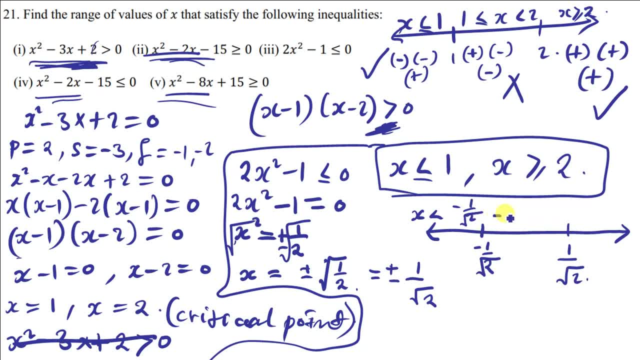 Here you have negative 1 over root 2 less x less 1 over root 2.. This side you have x greater than 1 over the root of 2.. So these are the regions that we have. Now let us test for the solution. 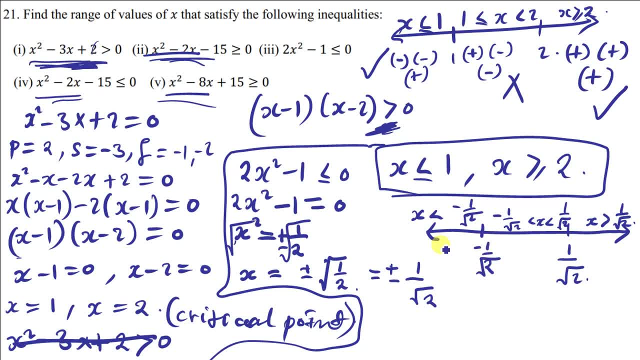 So any number that is less than negative, 1 over the root of 2, you can even get negative 3.. And when testing, you can use this same expression here. Yeah, so you can use this expression, You can get negative 3.. 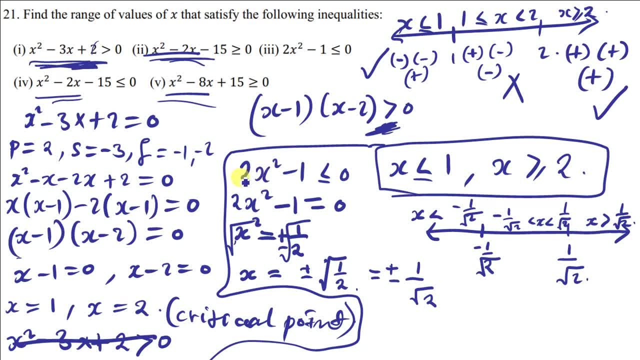 When you put negative 3 there, you are going to have 9 times 2.. That will be 18 minus 1.. 18 minus 1, that is 17.. Is 17 less or equal to 0?? The answer is no. 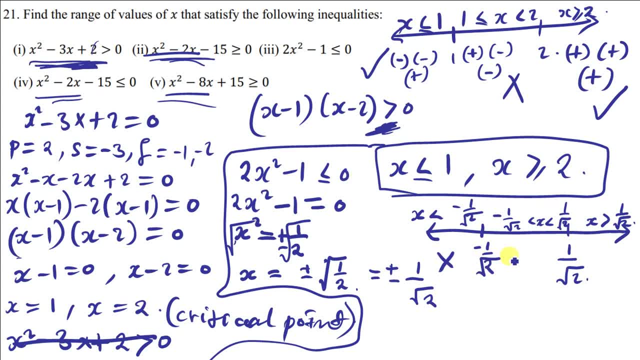 This region will be rejected. So we get any number that is between negative, 1 over the root of 2 and 1 over the root of 2.. We can even get a 0, because we know to say, between any negative and positive number, there is always 0.. 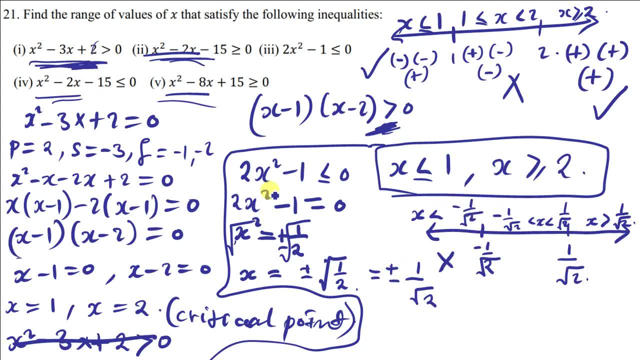 So we can get a 0. So when I put a 0 there, I am going to get negative 1.. Is negative 1 less than 0? The answer is yes, meaning this region will be accepted. Then you can also get any number that is greater than 1 over the root of 2.. 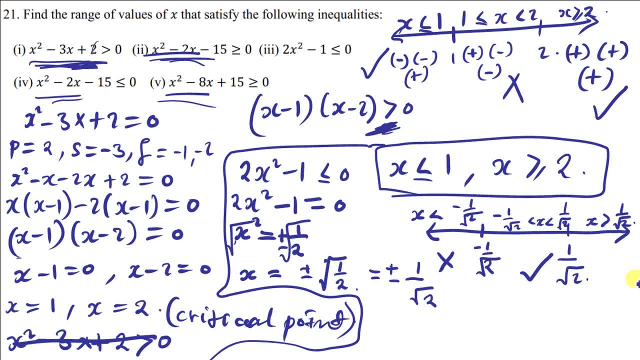 And that number. we can even get 2 or 3.. We can get 5.. Okay, let me use 5.. So 5 squared, the answer is 25.. 25 times 2, that is 50.. 50 minus 1, the answer is 49.. Is 49 less or equal to 0?? The answer is no. 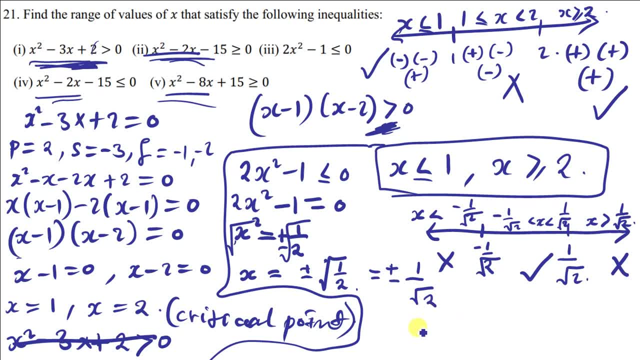 So this region is rejected. I mean, the range of values of x that we are looking for is simply just from negative 1 over the root of 2.. And because there is less or equal to symbol here, like I said, you put less or equal to symbols there. 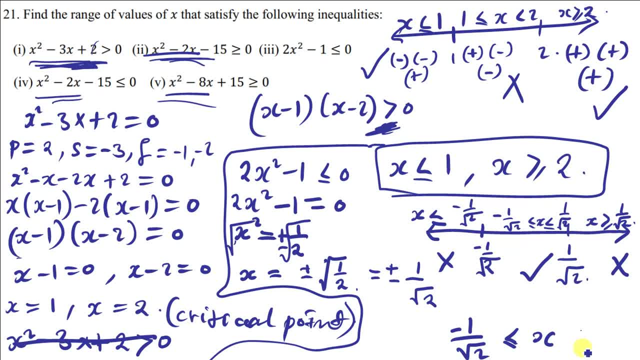 So we say less or equal to x, which is less or equal to 1 over the root of 2.. So this is exactly how you are supposed to solve such questions. So if you have any questions, feel free to contact me on any of the lines that I showed you on the screen. 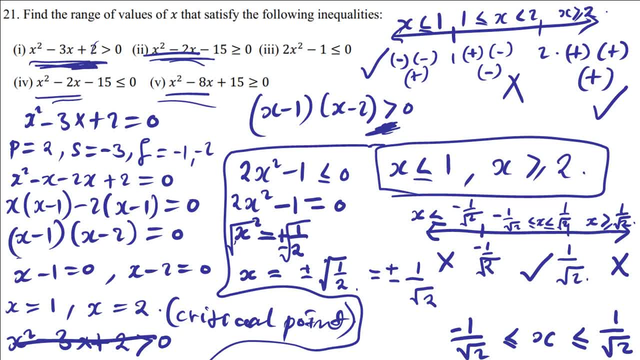 And don't forget to subscribe to the channel and also click on the notification button. My name is Hamtet. See you in the next tutorial video, Shalom shalom.